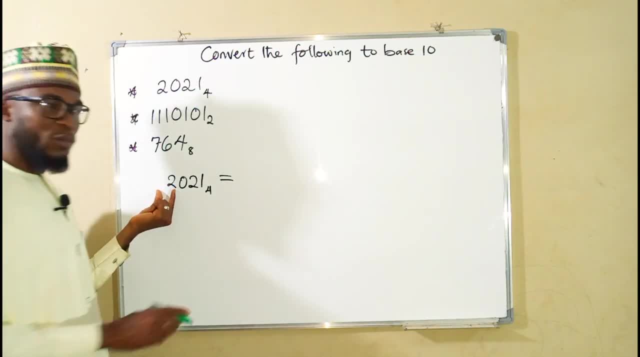 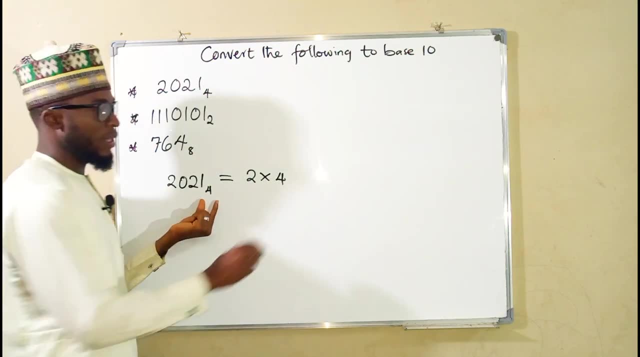 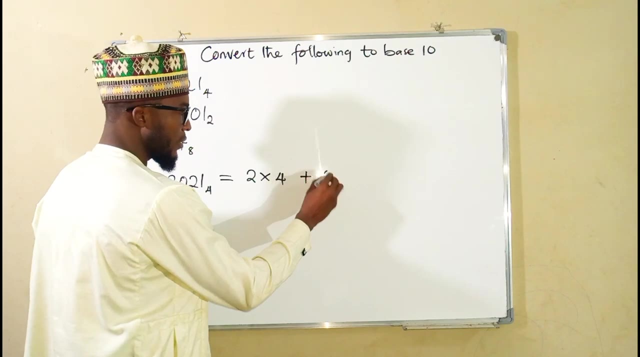 is how it is going to be. You take the first digit here, which is 2.. You multiply it with the base, and the base is 4.. You add, You take the second number which we have here as 0. You multiply it with the base, which. 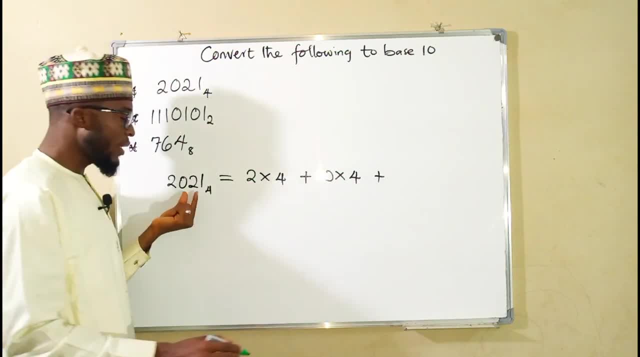 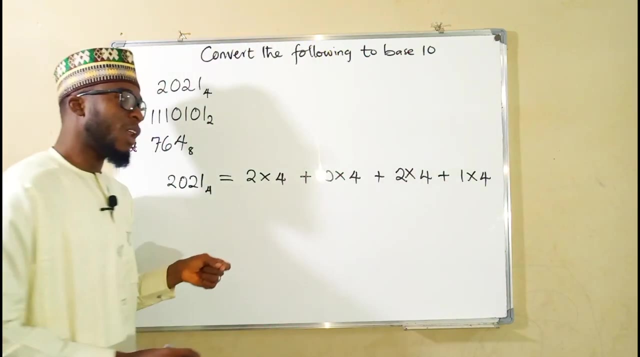 is 4. You add, You take the third number, 2. You multiply it with the base 4.. And lastly, we have: 1. You multiply it with the base, which is 4.. Having done this, we are going to assign. 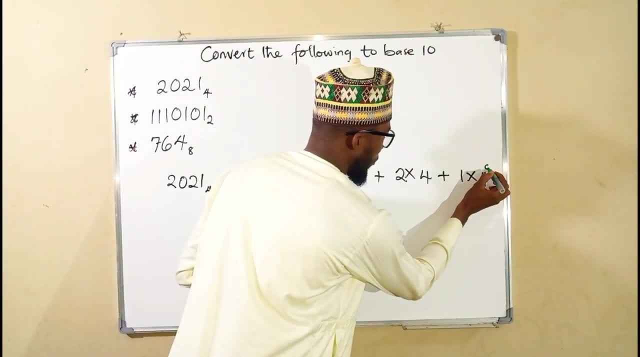 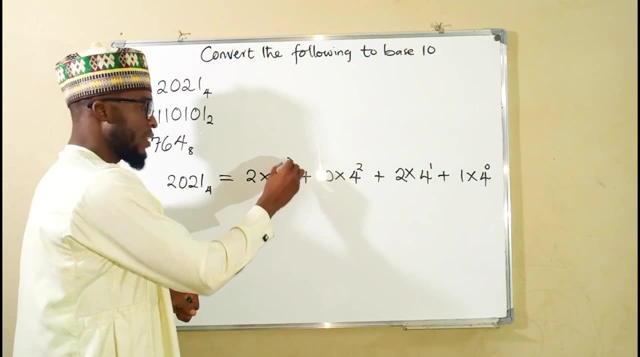 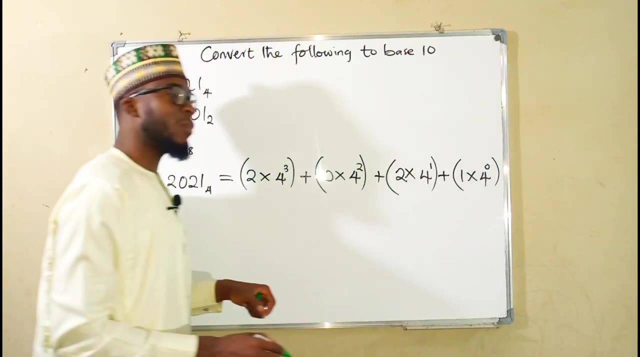 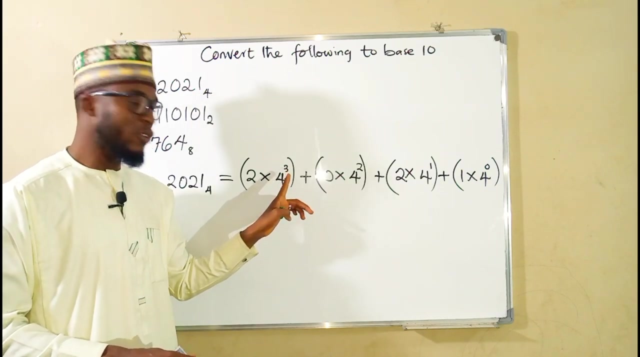 it to left with 0,, 1,, 2,, 3.. You stop, Then we are going to simplify these terms. What we obtain is going to be a number in base 10.. So we have 4 to the power of 3.. It does. 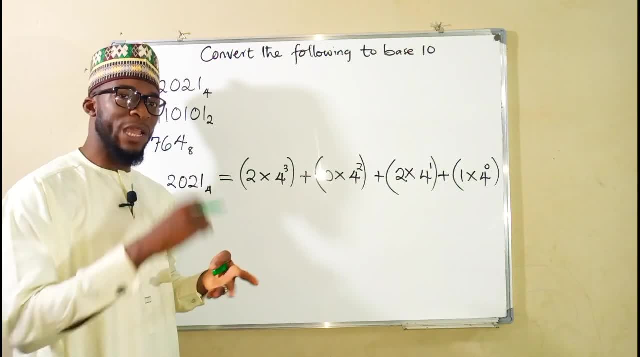 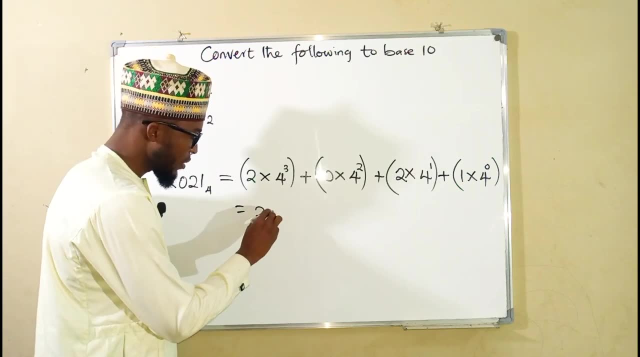 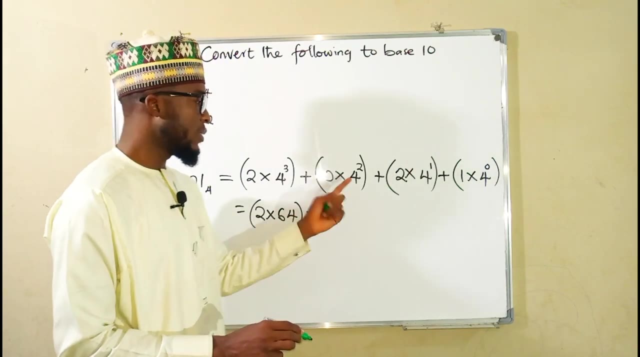 not mean 4 times 3.. It means 4 times 4 times 4.. 4 times 4 times 4 is 64. This is equal to 2 times 64. Plus 4 to the power of 2 meaning. 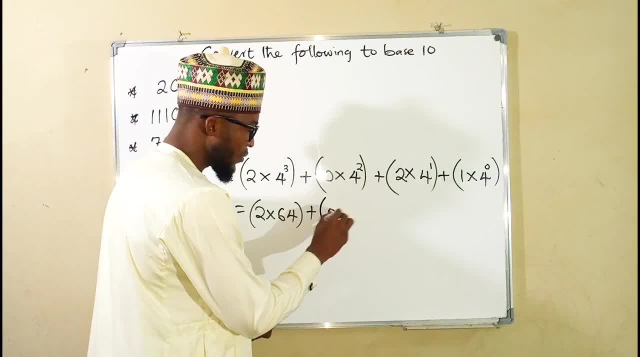 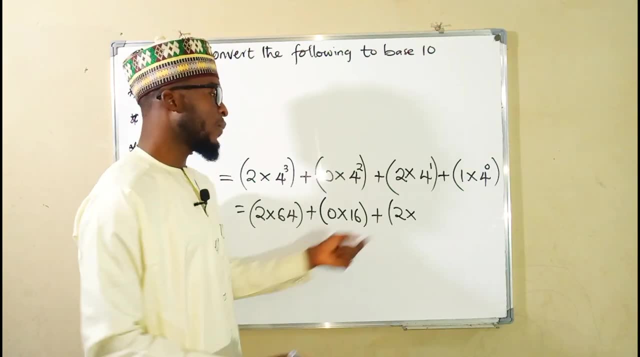 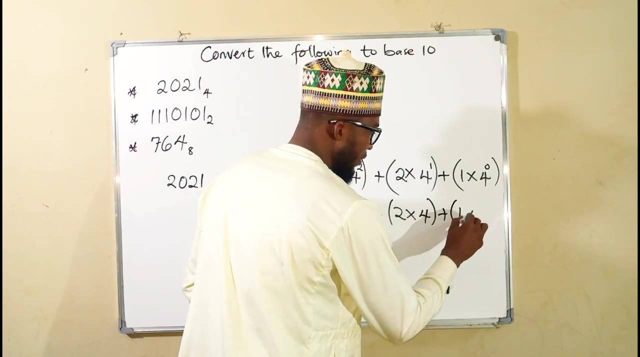 4 times 2 is 16.. So we have 0 times 16.. Plus 4 to the power of 1 is the same thing as 4.. Plus 1 times 4, power 0 is 1.. You know any number? power 0 is 1 except 0.. 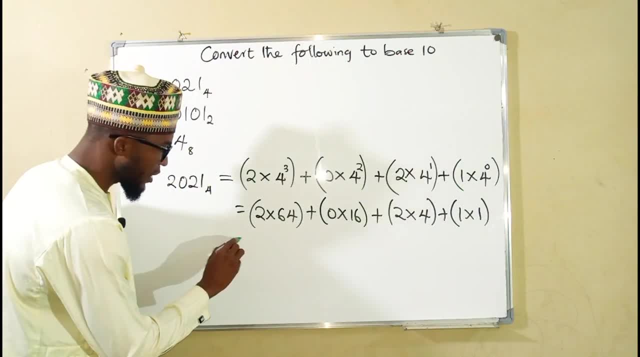 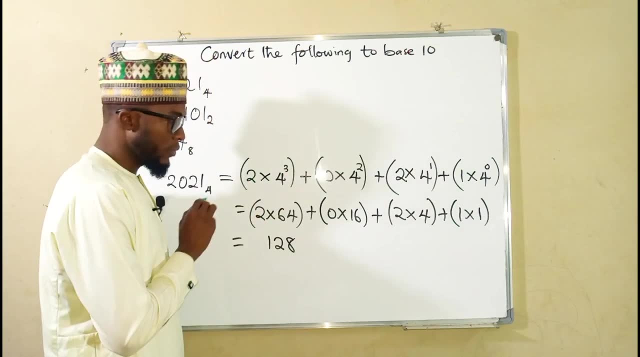 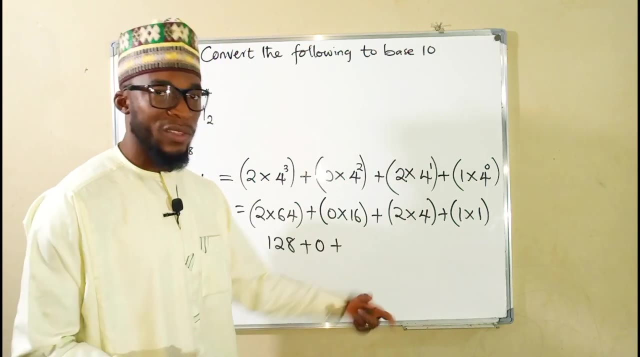 So this is 1.. We simplify for that again: 2 times 64 is 128.. Plus 0 times 16 is 0.. Plus 2 times 4 is 8.. Plus 1 times 1 is 1.. 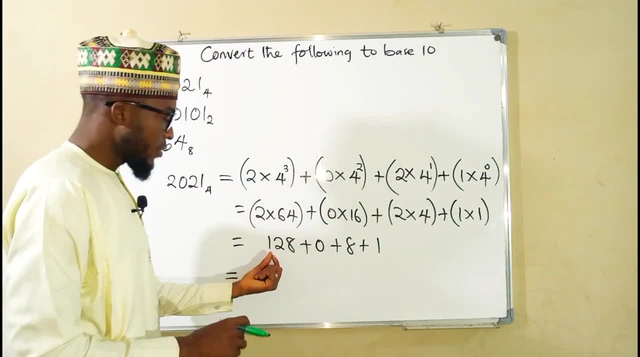 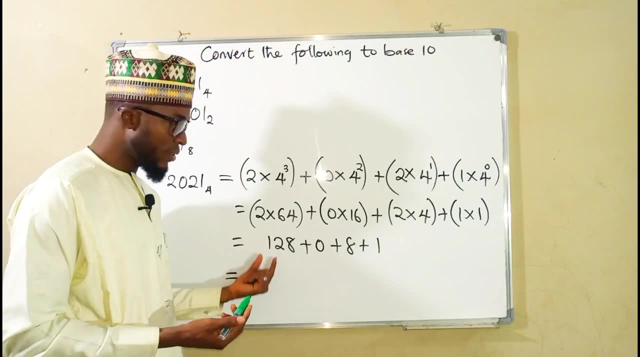 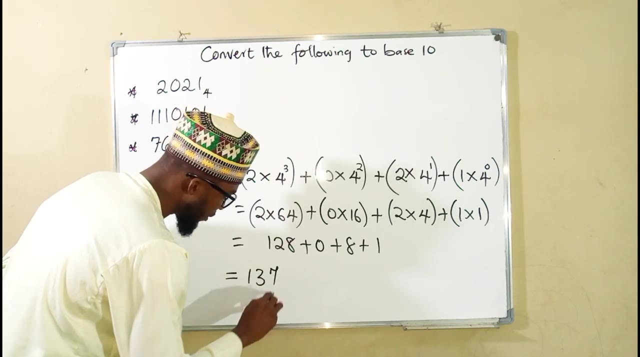 Then we add all this together: 128 plus 0 is still 128.. 128 plus 8 is 136.. And 136 plus 1 is 137.. So we have 137, but this number is in base 10.. 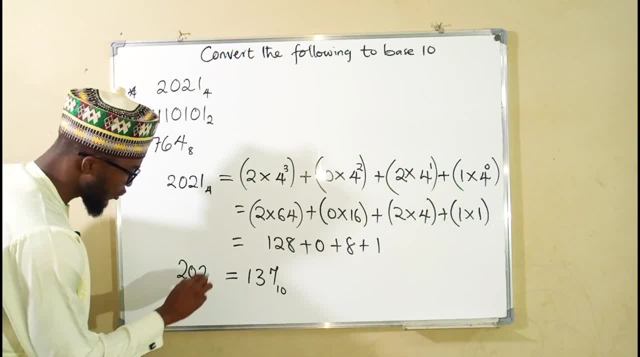 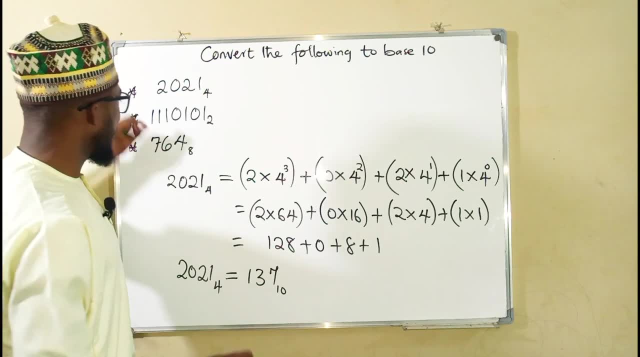 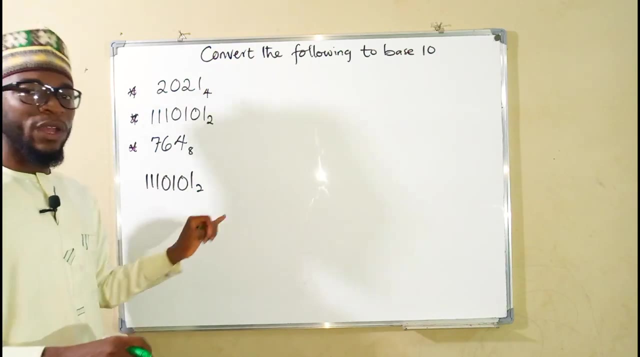 And hence you can see 20, 21 in base 4.. It is the same thing as 137 in base 10.. Now let us see how we can convert the second number here. So we have 1110101 in base 2.. 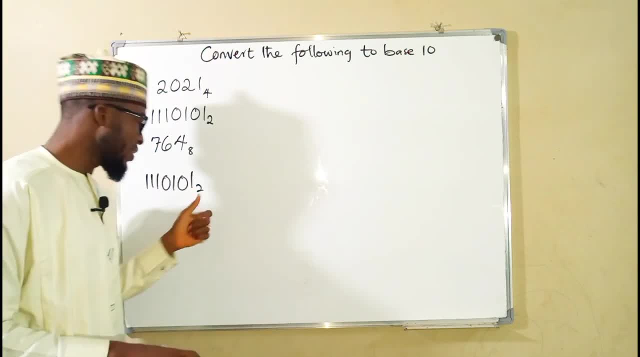 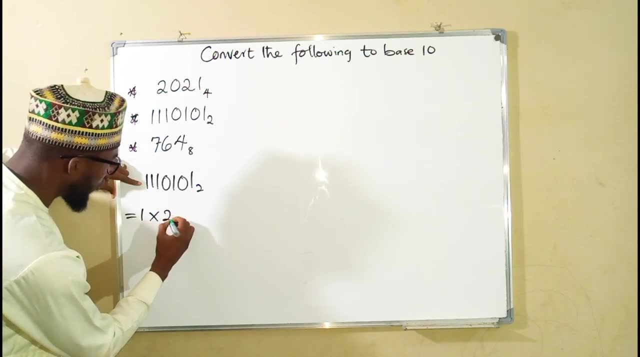 We are going to express it in powers of the base. The base is 2.. So we take the first number, which is 1, and we multiply it with this 2.. We add, We take the second number, which is 1, again times 2.. 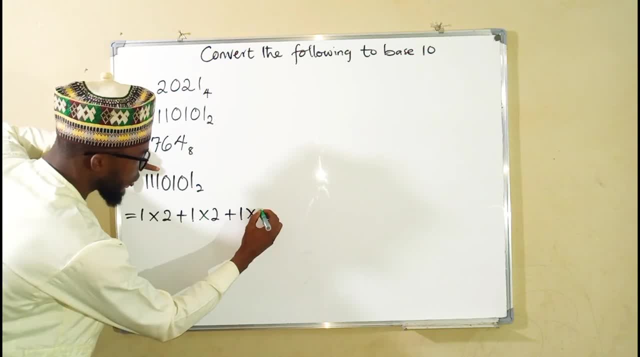 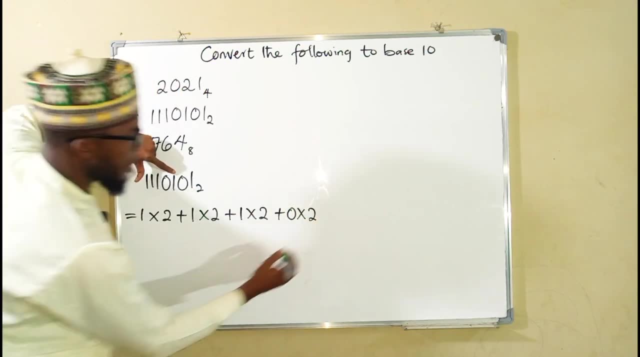 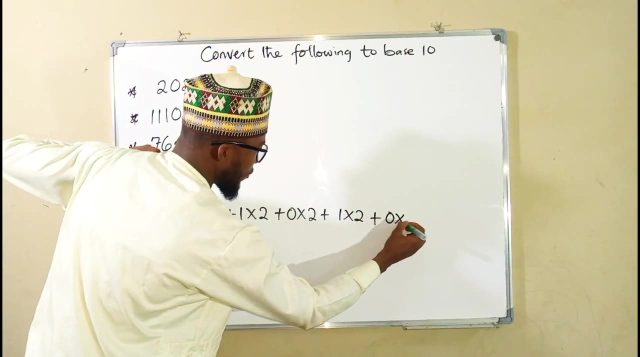 We add. We take the third number, which is also 1.. We multiply by the base. The fourth number is 0.. We multiply by the base. We have 1 times 2.. We have 0 times 2.. And, lastly, we have 1 times 2.. 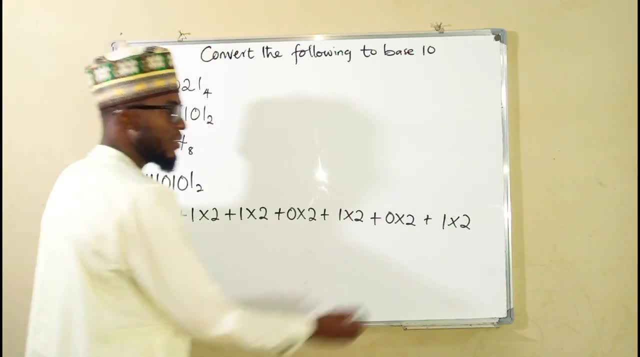 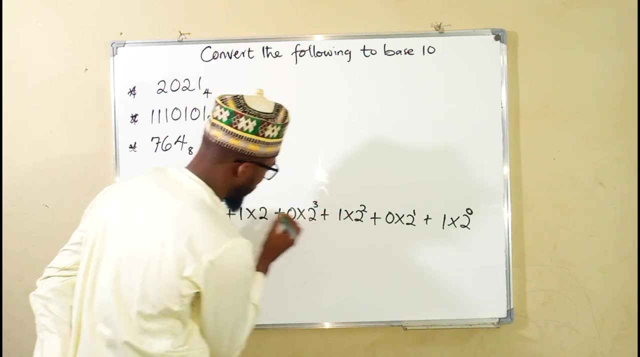 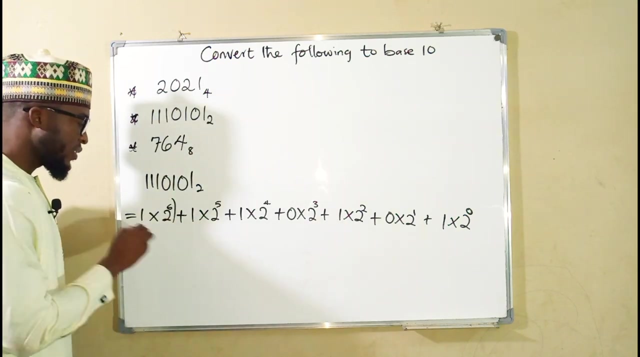 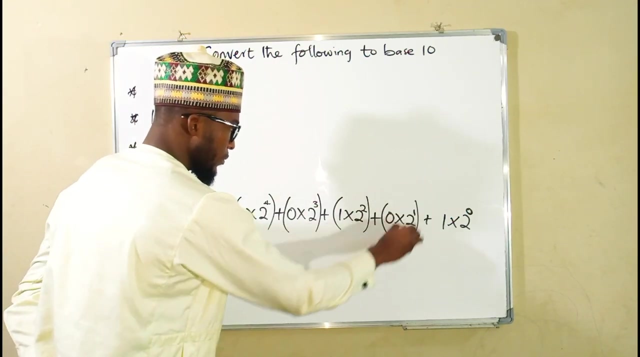 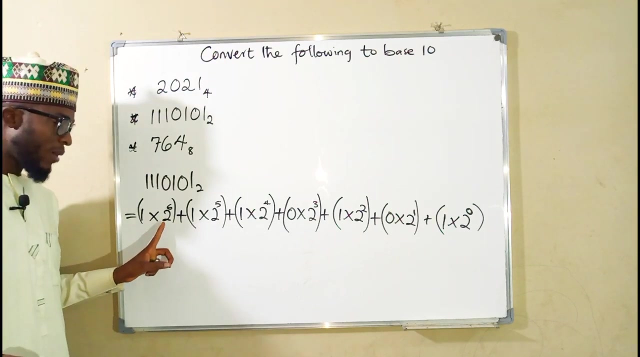 We are going to assign index to this basis, starting from 0, to the right Hand side: 0,, 1,, 2,, 3,, 4,, 5,, 6.. We are going to simplify each term, So here we have 2 to the power of 6, meaning. 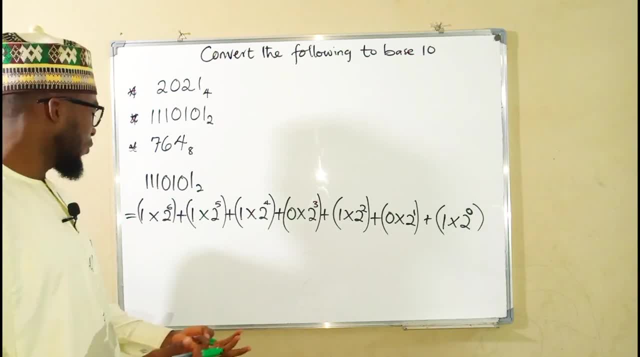 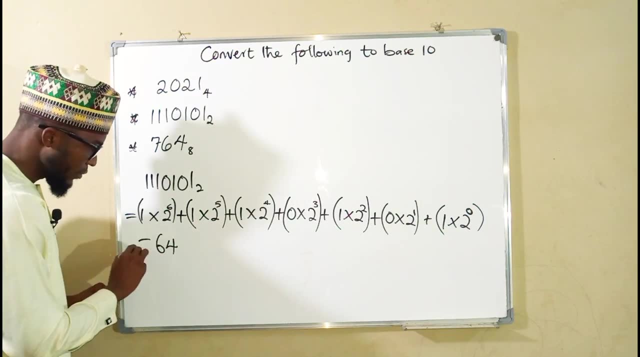 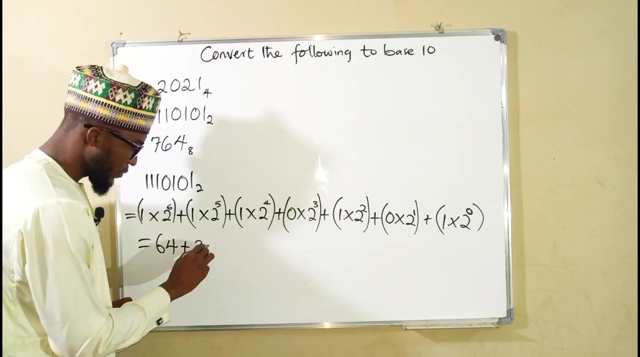 times 2, times 2, times 2,, 2 times 2 times 2, which is going to give us 64, and that 64 times 1 is still 64.. 2 to the power of 5 is 32,. 32 times 1 is 32 plus 2 to the power of 4 is 16, 16 times. 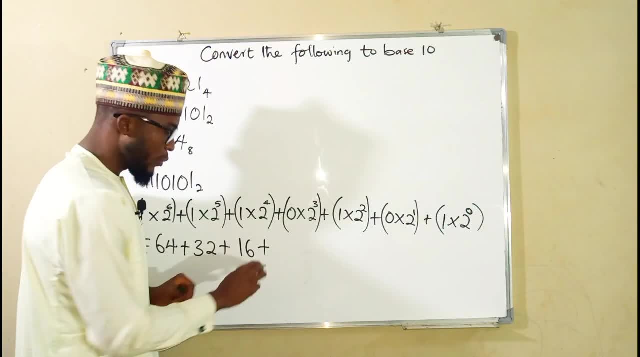 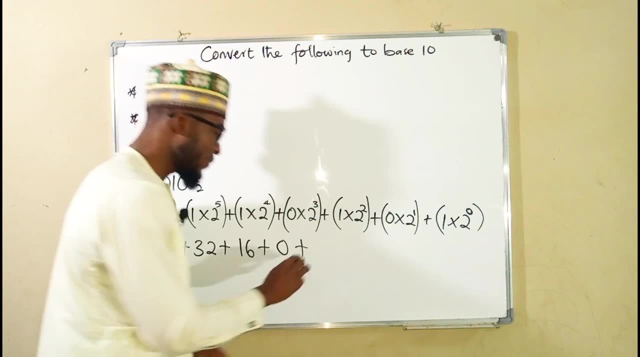 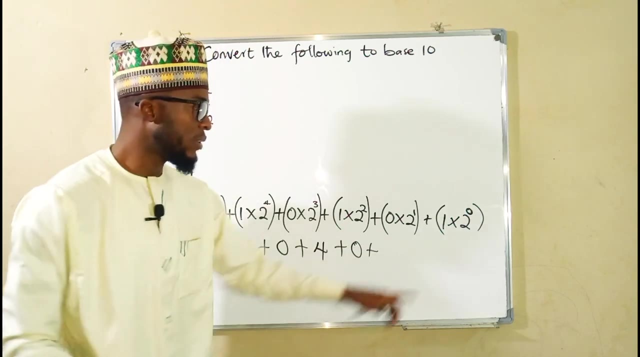 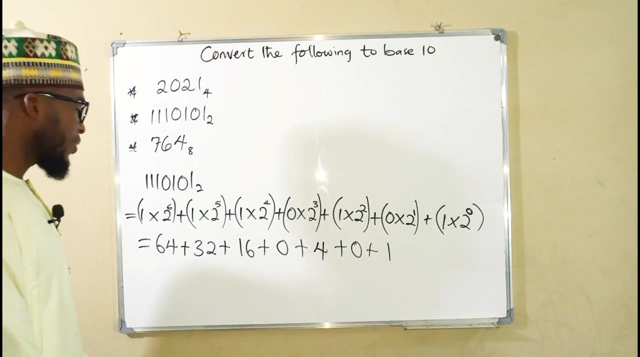 1 is 16 plus 0 times, this is going to be 0 plus 2. power 2 is 4 times 1 is 4 plus 0 times. this is going to make it 0 plus 2. power 0 is 1, then 1 times 1 is 1, then we add all together. 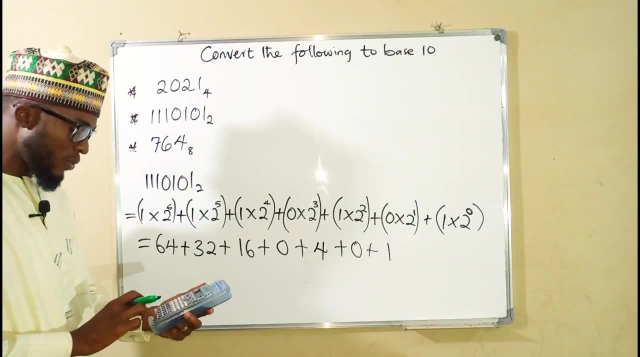 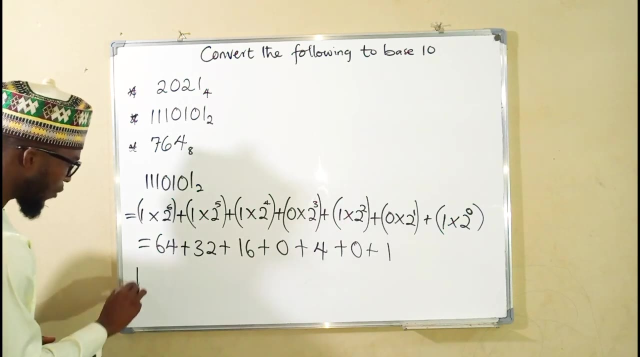 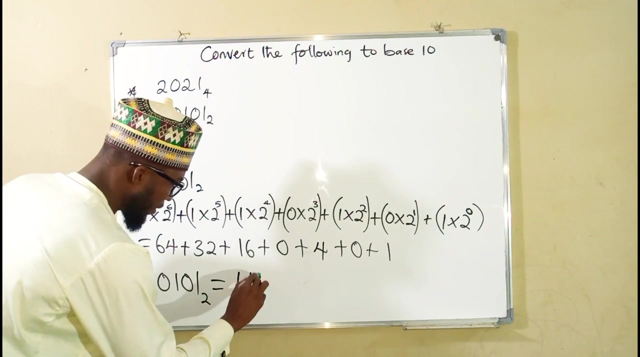 we have 64 plus 32 times 1 is 16.. Plus 16 plus 4 plus 1, we have all together 117, which is a number in base 10, and therefore 1110101 in base 2 is equal to 117 in base 10.. 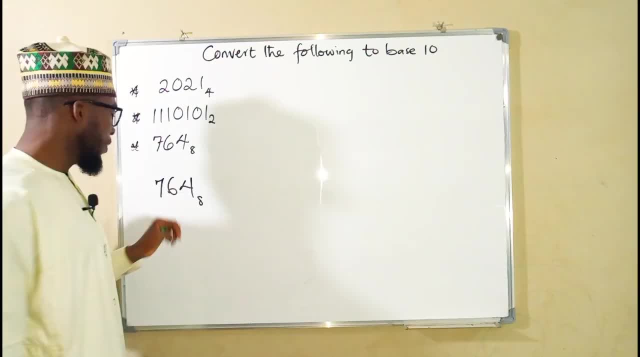 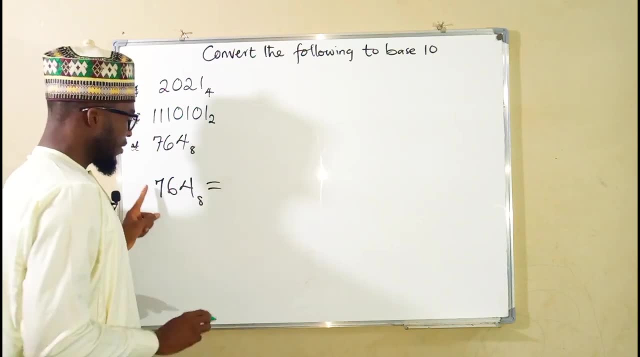 So now let us look on to the last one, which is 764.. We have 764.. We have 764.. We have 764 in base 8.. We are going to transform it in powers of the base. The first digit is 7.. 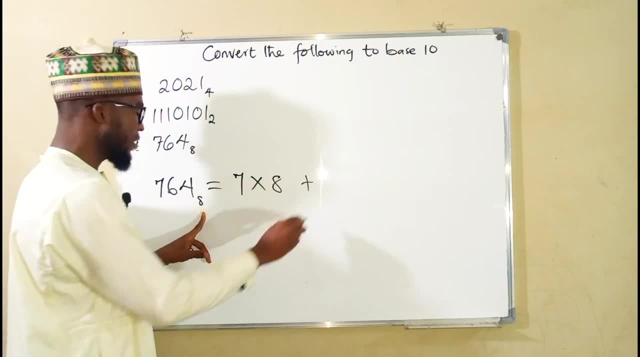 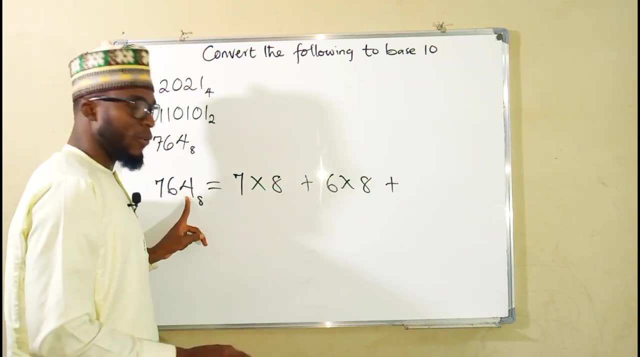 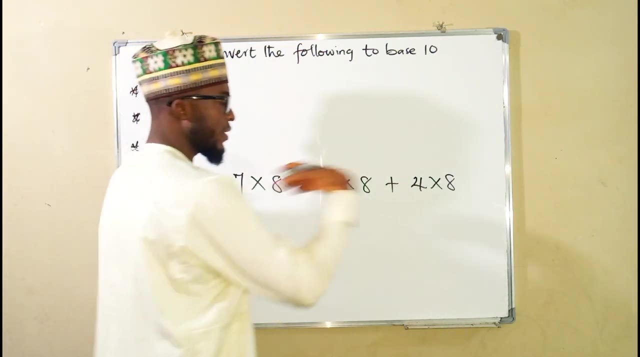 We multiply it with the base, which is 8.. We add, Take the second digit, which is 6.. You multiply by the base. You add, You take the last digit, 4.. You multiply with the base. We are going to assign index from the right to left, starting with 0,, 1,, 2.. 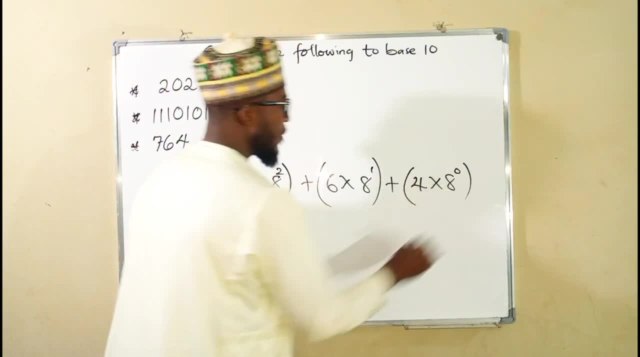 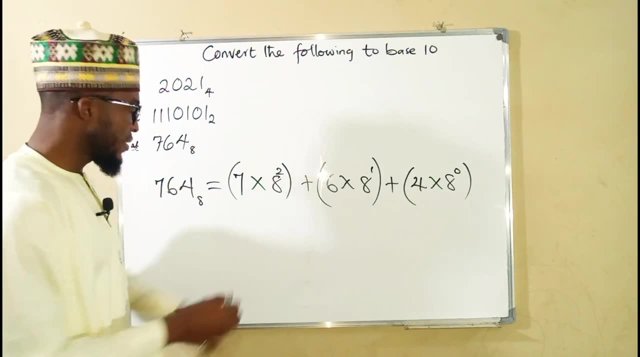 We are going to assign index from the left to left, starting with 0,, 1,, 2.. We are going to simplify. whatever we obtain is a number in base 10.. 8 power 2 is 8 times 8, which is 64.. 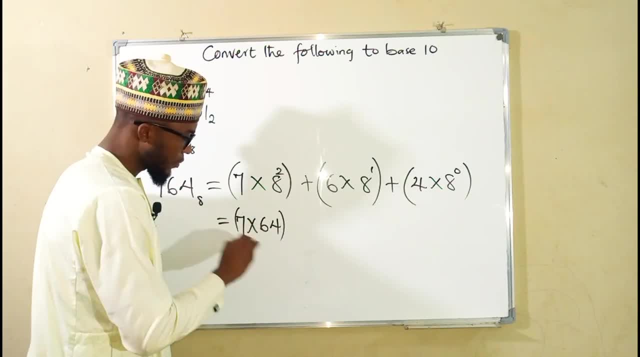 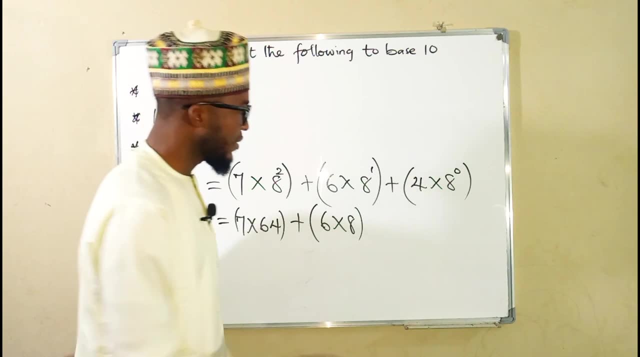 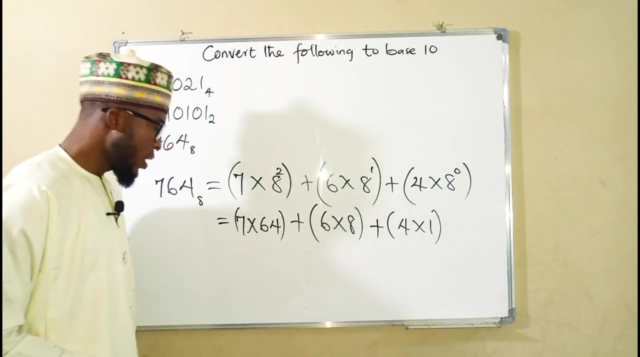 This is 7 times 64, plus we have 6 times 8, because 8 power 1 is the same thing as 8, plus the last one, which is 4 times 1, because 8 power 0 is 1.. So we have 7 times 64.. 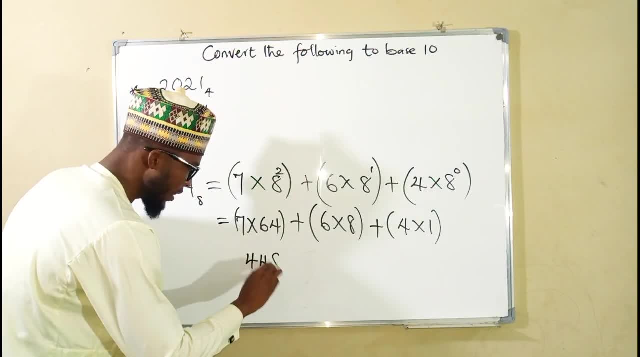 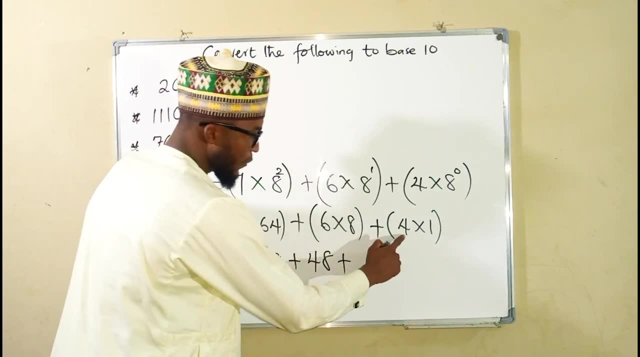 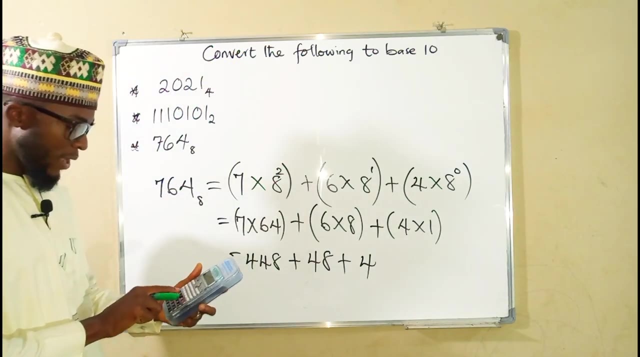 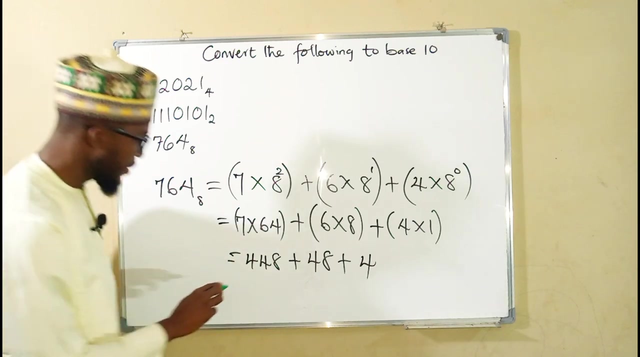 We have 448 plus 6 times 8 is 48 plus 4 times 1 is 4.. We add all of them together, We have 448 plus 4, 8 plus 4. altogether We have 500. So this is equal to 500 and this 500 is a number in base 10.. 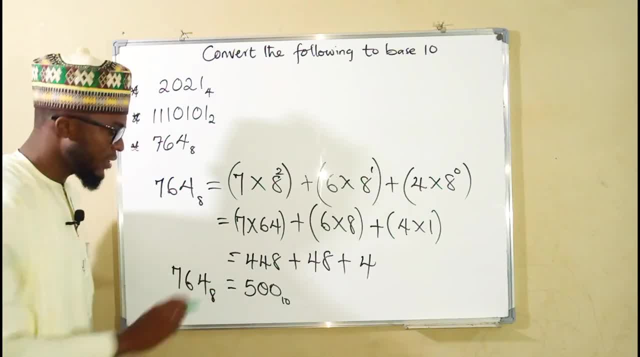 And hence we say: 7,, 6,, 4 in base 8 is equal to 500 in base 10.. And this is all I have for you today. Thank you for watching. Do have a nice day.